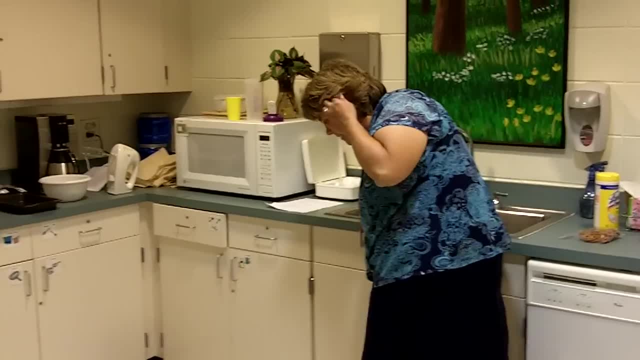 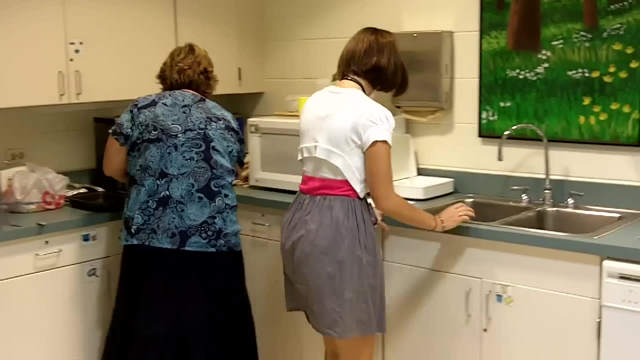 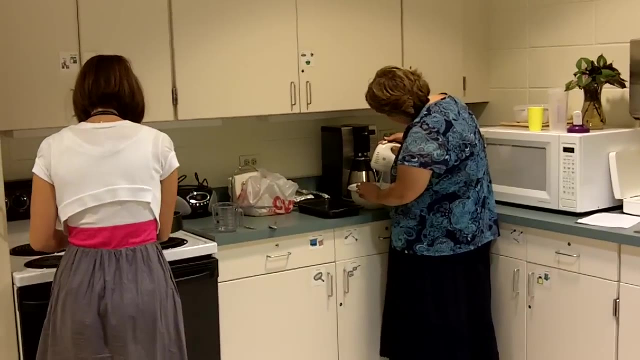 Whoa, it's slippery. That's it on the floor. Okay, Chef, make sure you step over there. Kind of slippery, I don't have time to clean it now. Okay, Love brownies. Oh, something's not right here. 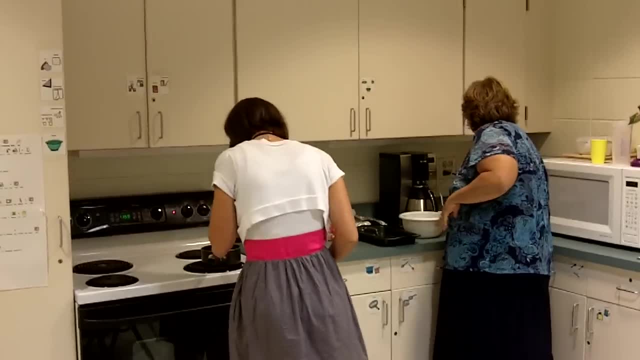 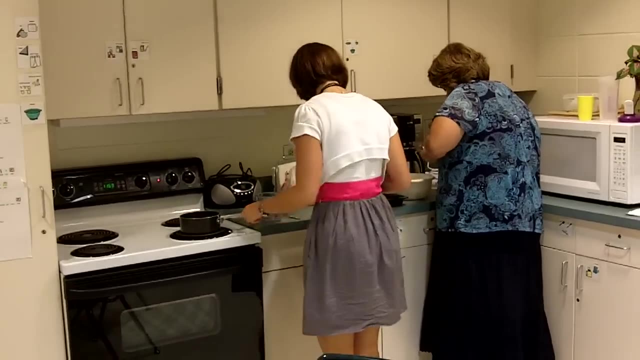 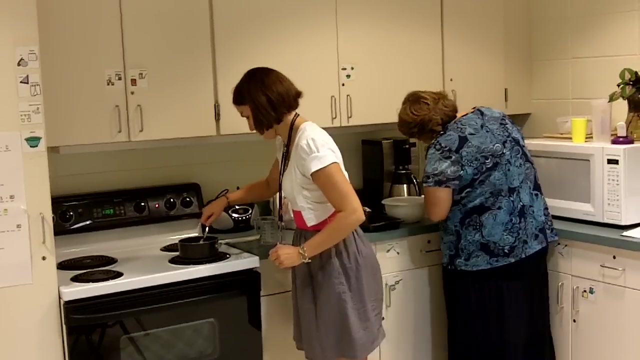 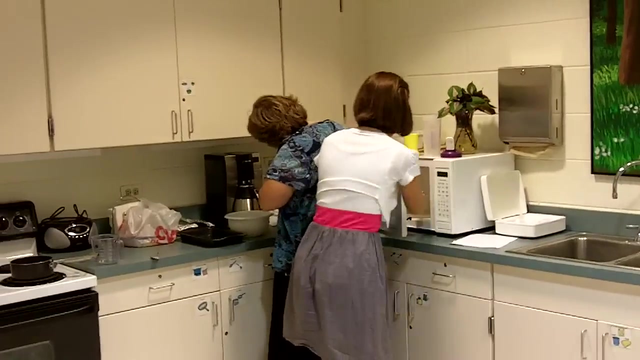 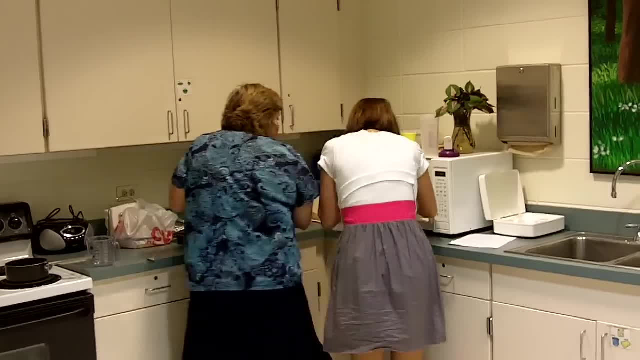 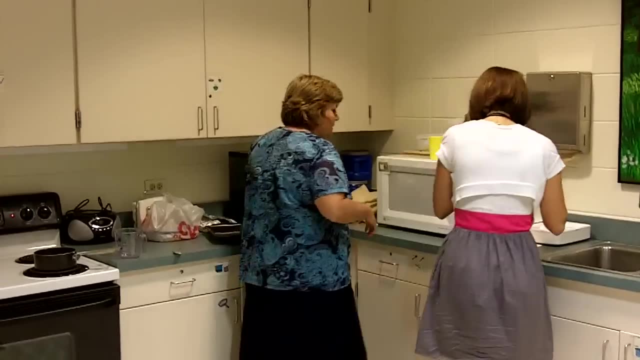 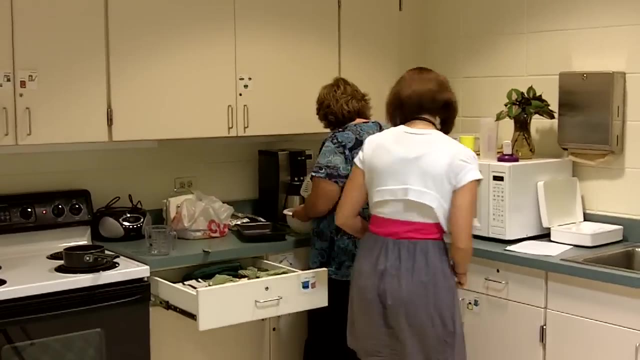 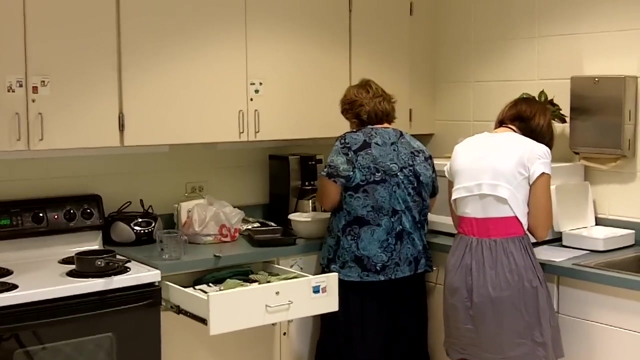 Oh, oh, oh, That's good, Here we go. Oh, oh, oh, oh, I think this is our. Hmm, Huh, sparks in the microwave. okay, let's see here. next on the recipe: let's see, oh I. 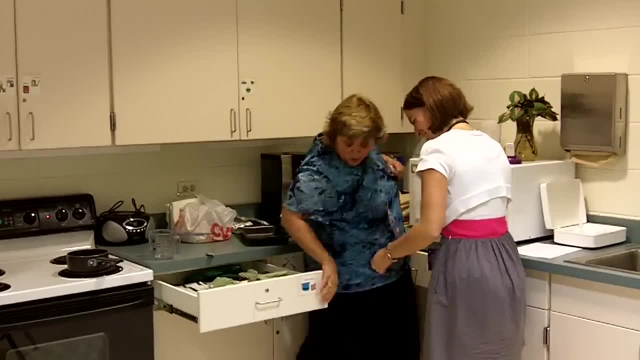 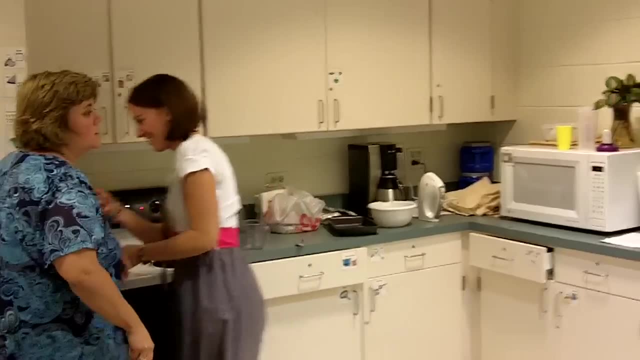 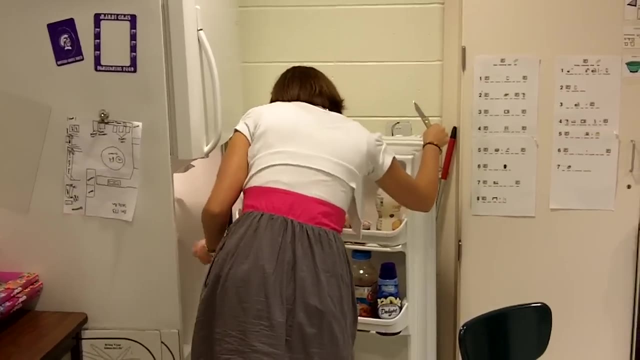 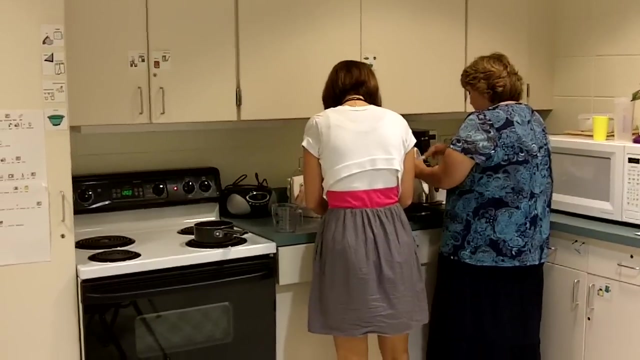 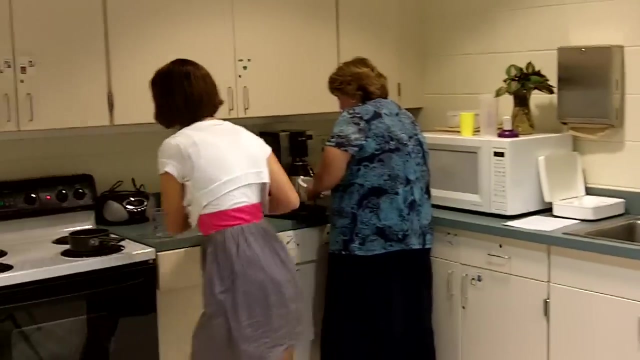 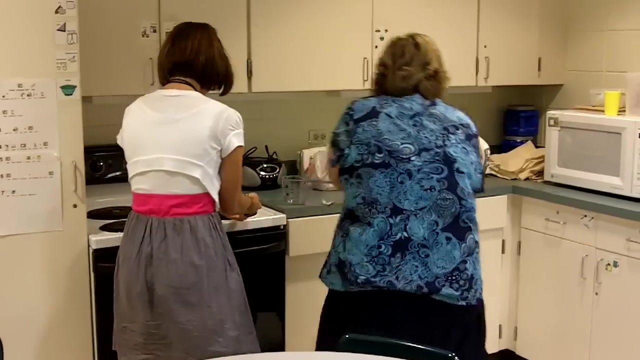 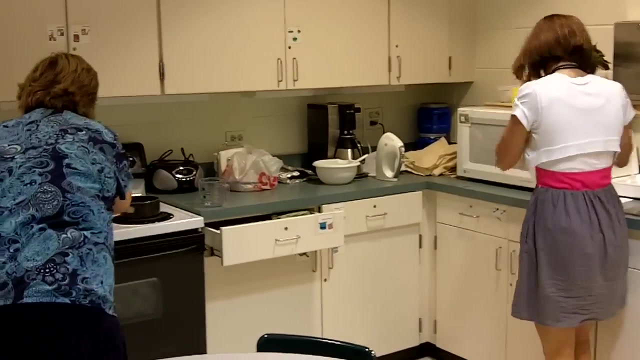 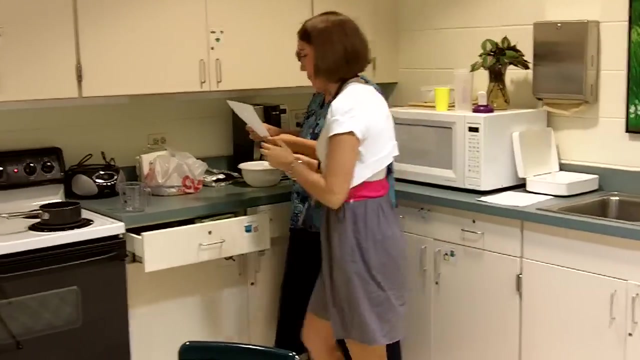 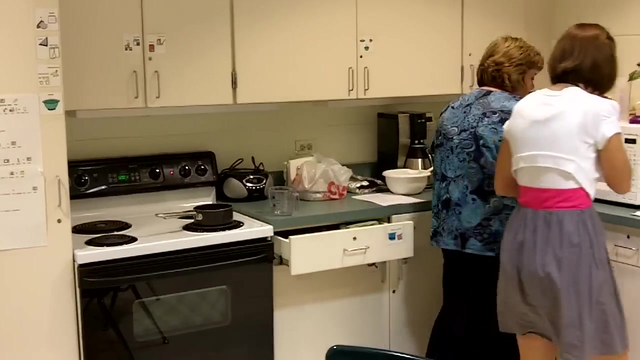 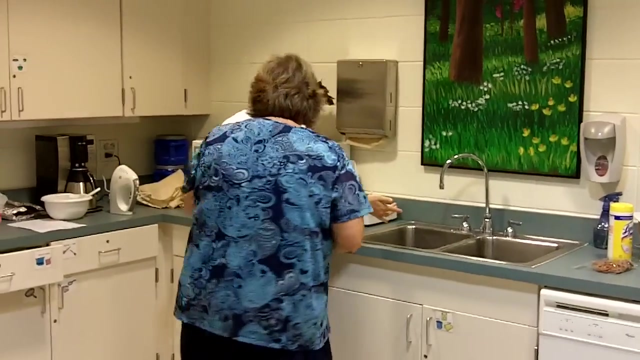 know what I need. you make the butter. watch out, that's a nice, really sharp, really sharp. go burn here, Sally, careful. let's see what do I need next? let's taste this cheese. really good, you can use this to cut the brownies, okay, are you? okay? I'm sorry, I. 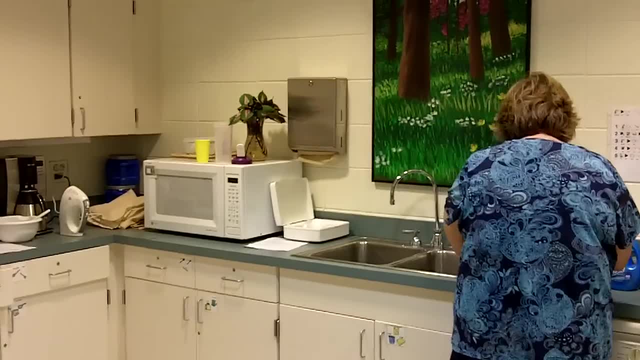 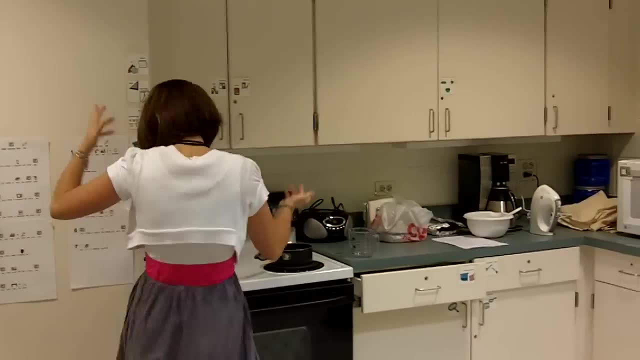 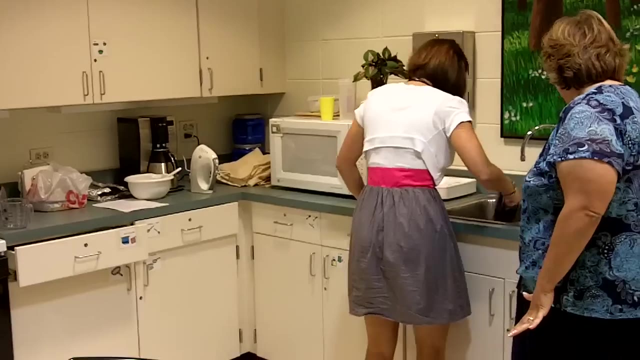 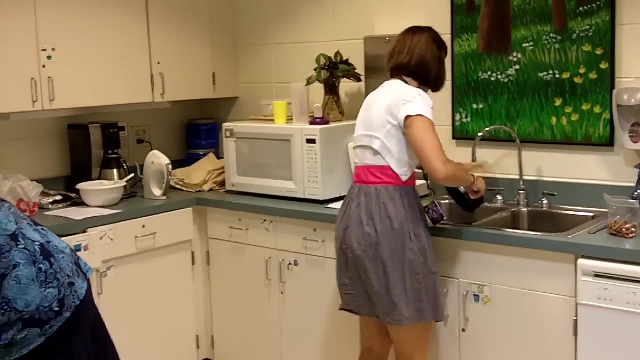 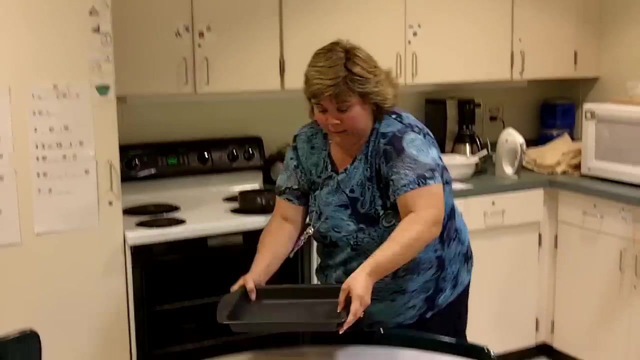 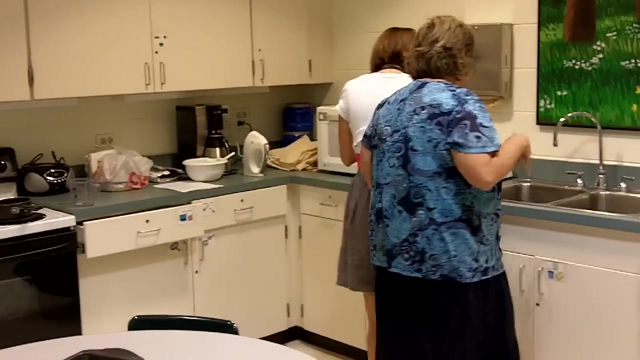 didn't need to do that. yes, why is it so slippery? it's done. hey, there's some pretzels over here. oh, okay, I should wash this right away, right away. oh geez, third degree burn right now. okay, I think I'm just about. I think, if you. 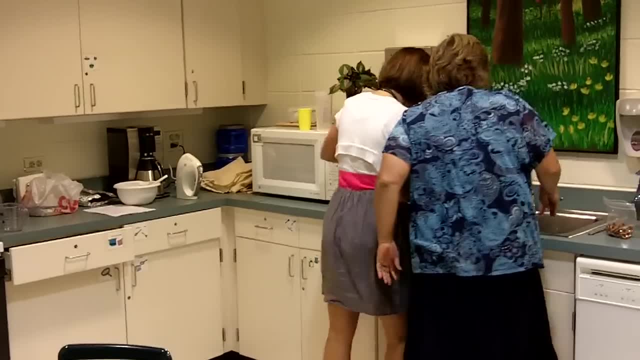 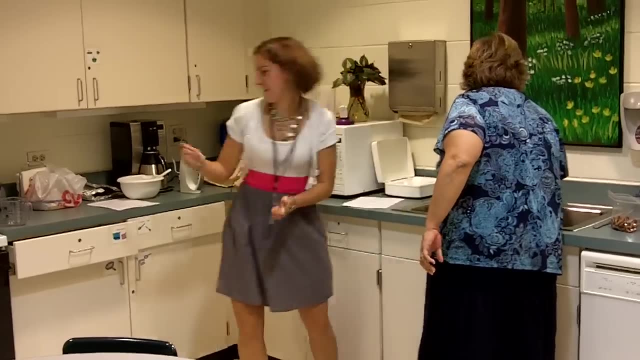 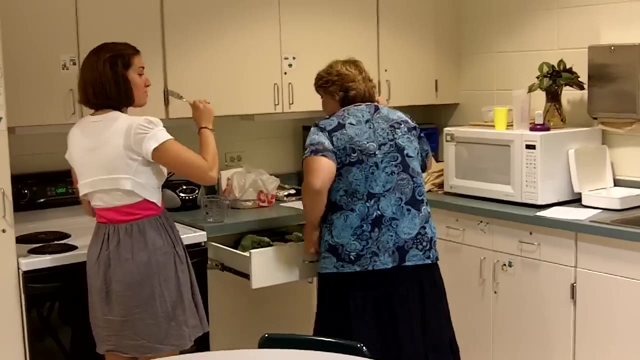 put your hand in hot water, I'll feel better. maybe it was cold water. wait, I gotta mix. I gotta mix my mac and cheese. this is clean. is this a little clean? lets mix this mac and cheese. it's delish, excellent. I can't wait to have some. 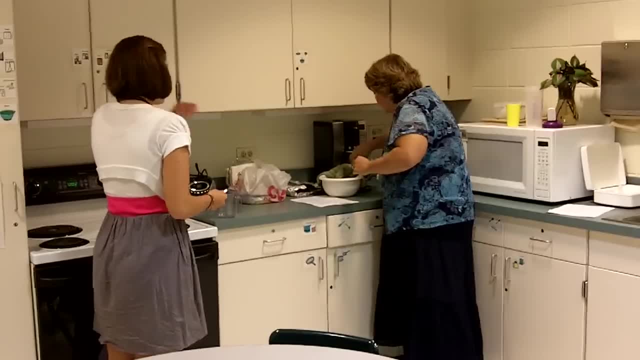 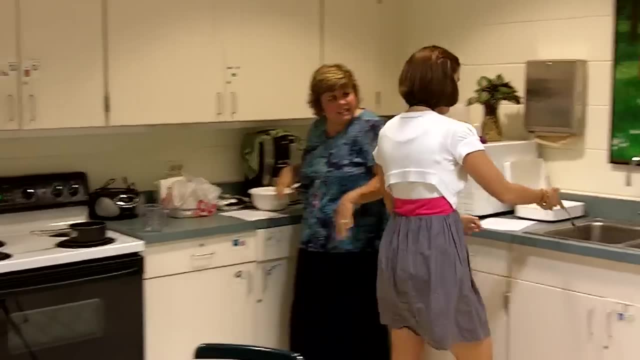 okay, let's just feel the. oh, it went in the brownies. taste. test it good, mac and cheese tasty, very, very okay, wait, I think I'm just about done here. it's starting to burn. I'm gonna try some more. okay, I think I'm just about done here. it's starting to burn. I think I'm just about done here. it's starting to burn. I'm gonna try some more. 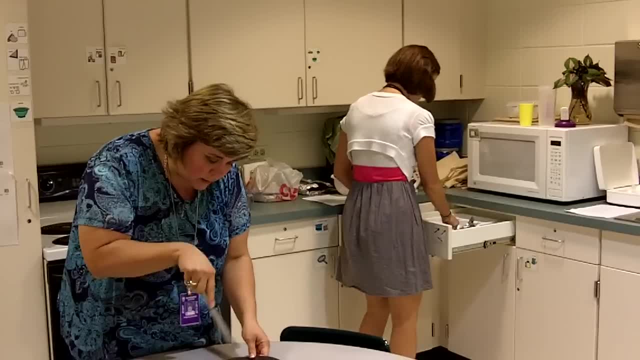 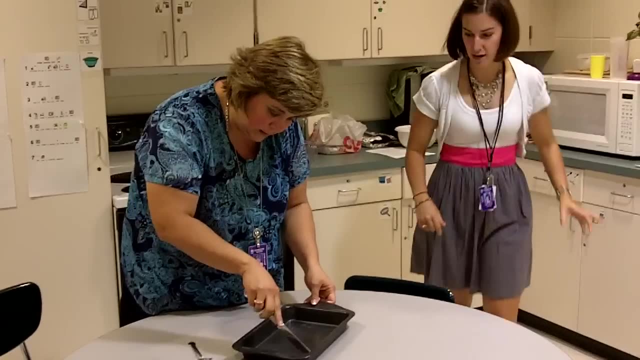 Oh, sorry, That's okay. Okay, How are the brownies? They're looking good, Mmm, Mmm, Very fudgy, Very. Oh, oh You know what. Maybe I should put them back in. Maybe I should put them. 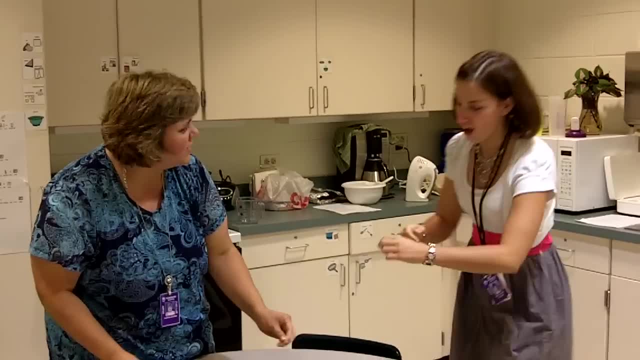 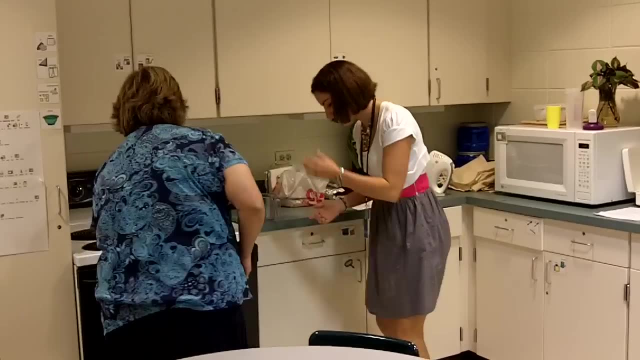 There they are. I like them kind of not done. Boozy, goozy, Whew, This is really slippery. What is going on here? I don't know, It's dirty too. Okay, Okay, Okay, Okay Okay. 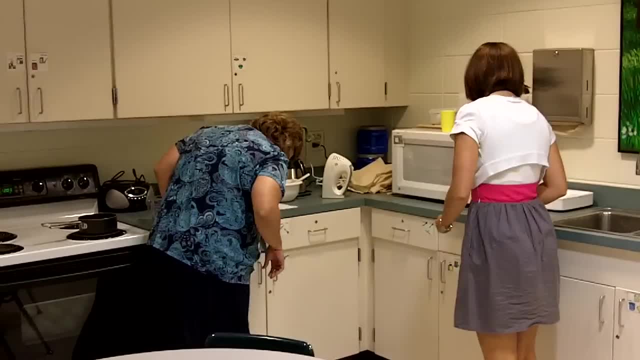 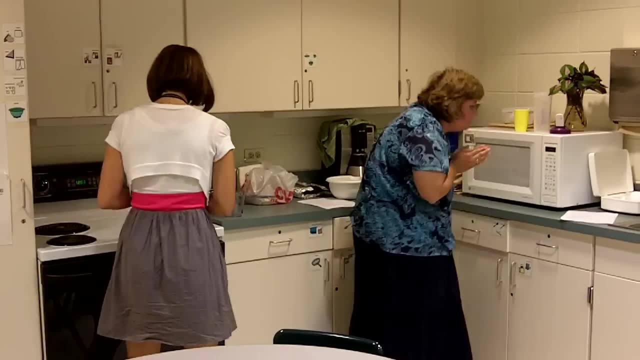 Okay, Okay, Oh my God, Oh my God, Okay, Okay, Oh my God, It's dirty too, Okay, Achoo, Bless you, Bless you, Okay, Okay. You know what This was? just noodles in here. 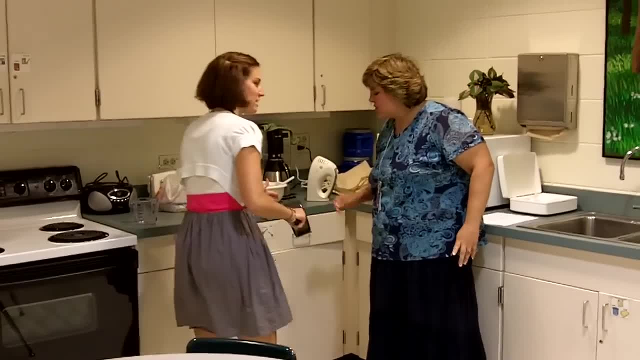 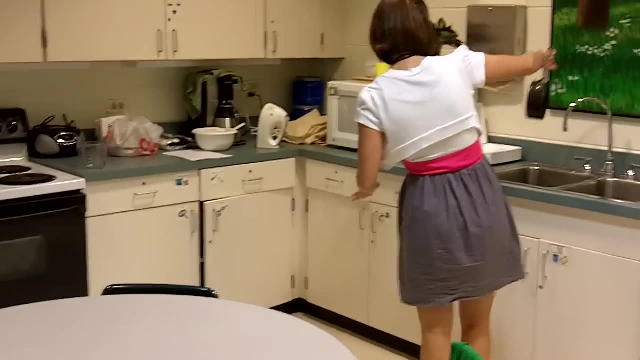 I don't think it's that dirty. I might put it back or something. You know what. Just rinse it out. Oh, just rinse it. Just rinse it, Quick rinse. That looks good, Okay Let's. Oh, it's steaming.